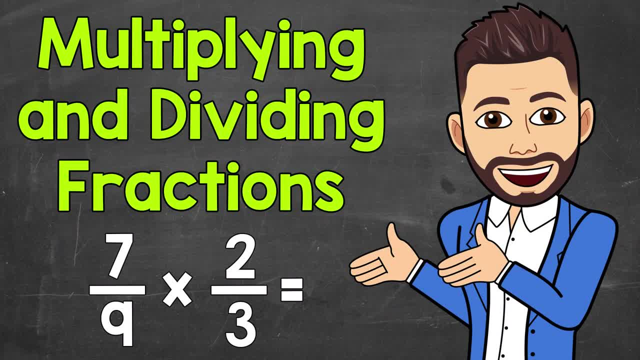 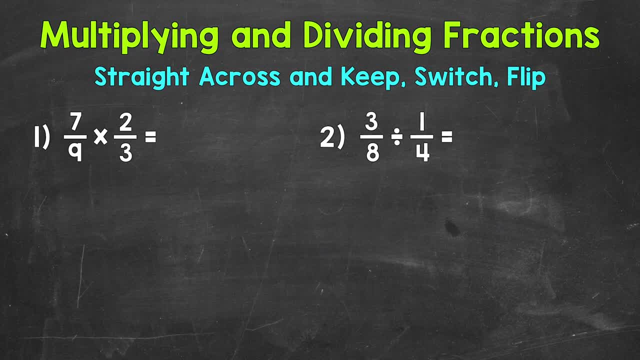 Welcome to Math with Mr J. In this video I'm going to cover how to multiply and divide fractions. We'll go through one example each and I'll explain each step as we work through the problems. Let's jump into our examples, starting with number one, where we have seven. 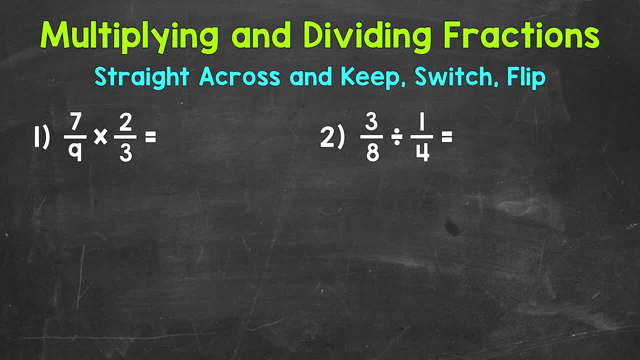 ninths times two thirds. Now when we multiply fractions we multiply straight across. So numerator times numerator, the top numbers in our fractions, and then denominator times denominator, the bottom numbers in our fractions. So let's start with the numerators Seven. 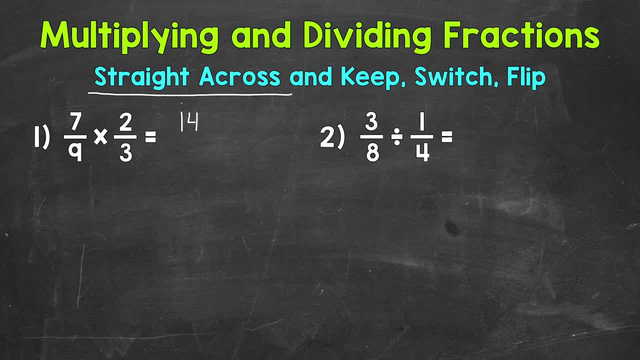 times two, that gives us fourteen. Our denominators nine times three, that gives us twenty-seven. So our answer is fourteen, twenty-sevenths, Always. look to see if you can simplify, but in the case of number one, The greatest common factor between fourteen and twenty-seven is one. That means we are. 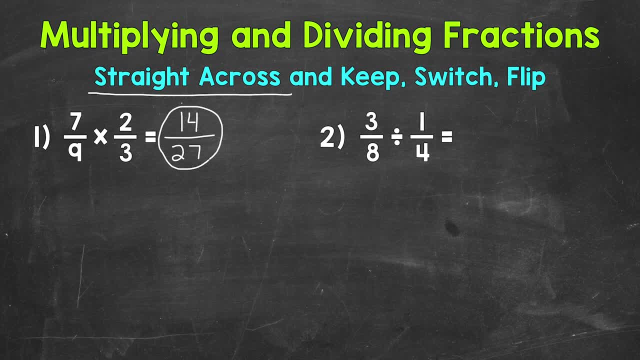 in simplest form and done with the problem. So final answer for number one: fourteen, twenty-sevenths, And again, when we multiply fractions, multiply straight across. Let's move on to number two, where we have three eighths divided by one fourth. Now, when we divide fractions, we keep 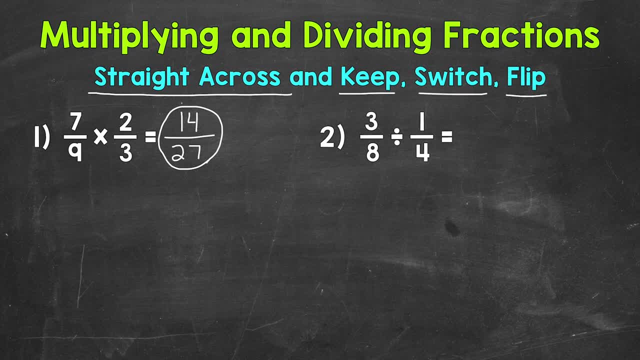 switch flip. You may also hear keep, change, flip. They both mean the same thing. So I'm going to rewrite the problem using these steps. So keep, always keep your first fraction, So three eighths. Then our next step is switch. We are going to switch from division to multiplication. 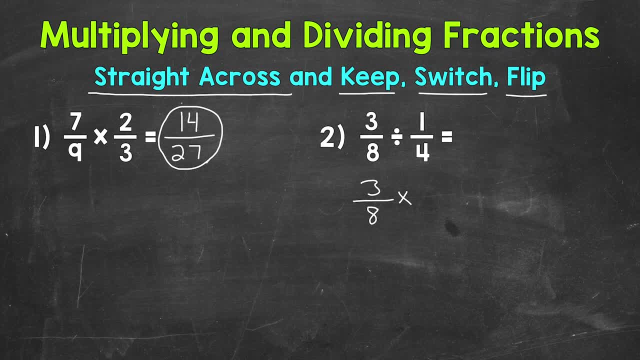 So let's switch this to multiplication. Multiplication is the opposite of division. So our last step is flip. we are going to flip our second fraction. This is called the reciprocal. So the 4 is going to be our numerator now and the 1 is going to be our denominator. 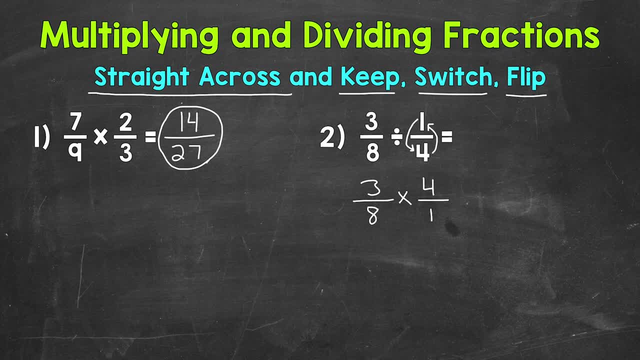 So we flipped that second fraction. Now we can multiply straight across: 3 times 4 is 12.. 8 times 1 is 8. We get 12 eighths, which is an improper fraction. So we want to convert this to a mixed number. 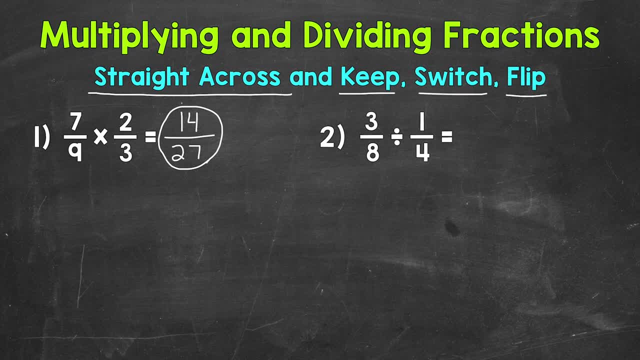 switch flip. You may also hear keep, change, flip. They both mean the same thing. So I'm going to rewrite the problem using these steps. So keep, always keep your first fraction, So three eighths. Then our next step is switch. We are going to switch from division to multiplication. 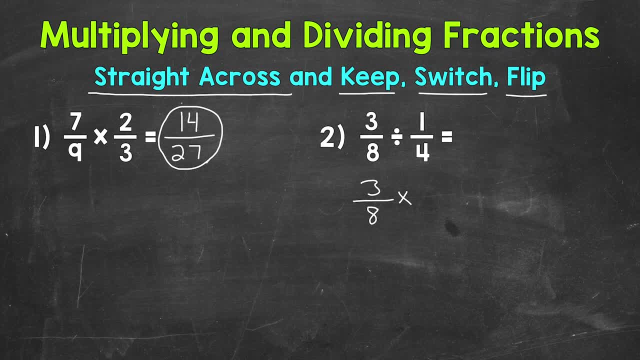 So let's switch this to multiplication. Multiplication is the opposite of division. So our last step is flip. we are going to flip our second fraction. This is called the reciprocal. So the 4 is going to be our numerator now and the 1 is going to be our denominator. 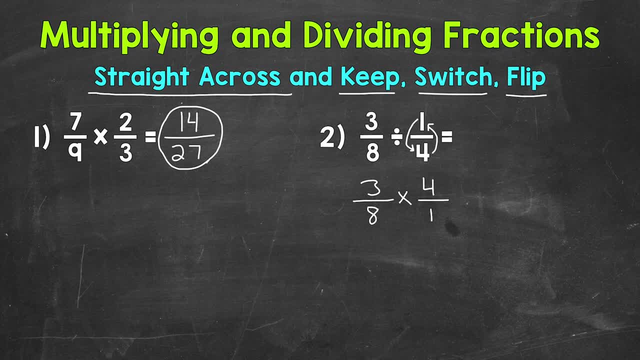 So we flipped that second fraction. Now we can multiply straight across: 3 times 4 is 12.. 8 times 1 is 8. We get 12 eighths, which is an improper fraction. So we want to convert this to a mixed number. 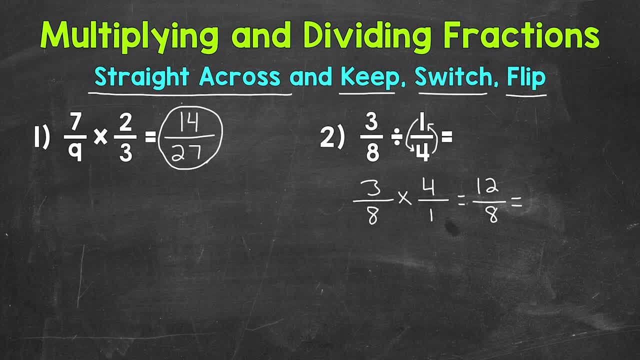 We do that by doing 12 divided by 8.. So how many whole groups of 8 can we pull out of 12? One whole group of 8.. That's our whole number. Now we don't hit 12 exactly. We have a remainder of 4.. 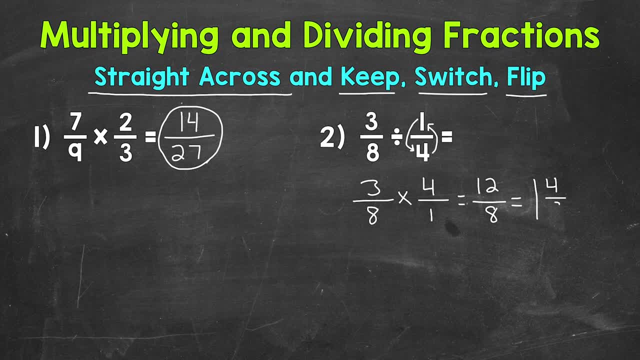 That's our numerator And we keep our denominator of 8 the same. So we get 1 and 4 eighths. Now that can be simplified. We have a common factor other than 1, between 4 and 8.. 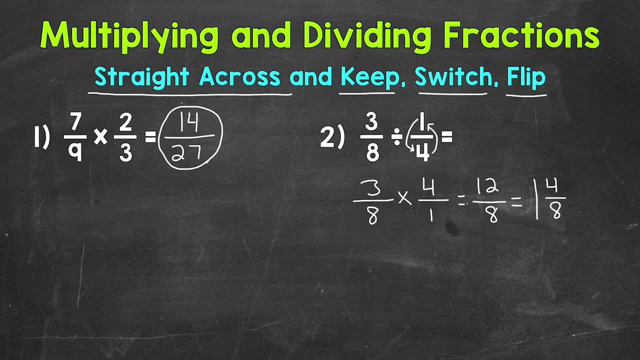 So we can put this into simplest form: Our greatest common factor is 4.. Let's divide both of these by 4. And we get 1.. 4 divided by 4 is 1., And 8 divided by 4 is 2.. 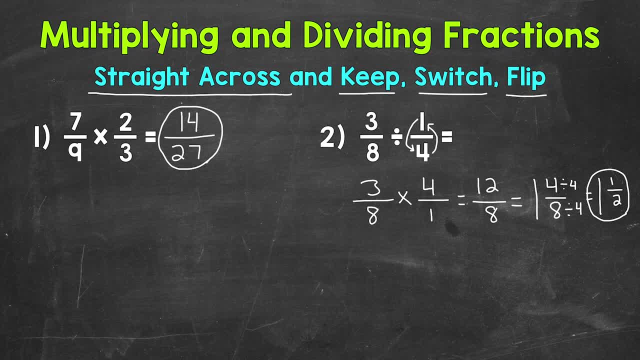 So we get 1 and a half for our final answer. So there you have it. There's how you multiply and divide fractions. I hope that helped. Thanks so much for watching. Until next time, peace.